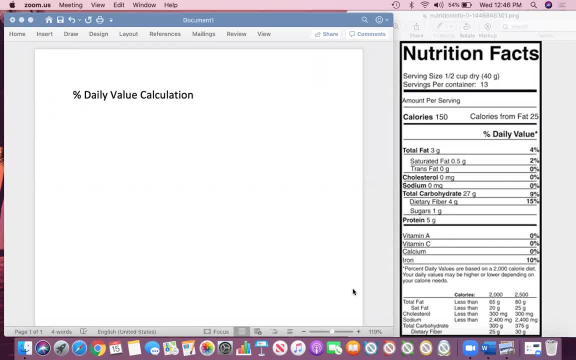 the percent daily value calculation for carbohydrates rather than fat. but then for the actual food labels assignment you will do the percent daily value calculation for fat. So on this food label here you can see that their total carbohydrates content in grams is 27 grams and you can see here that the 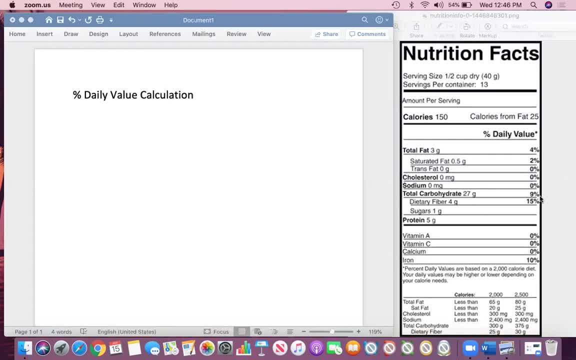 percent daily value listed on the food label is 9%. So just because it's listed on the food label, you could just write 9%, but you need to show your work in order to get full credit for this question. So to do that, you'll have to know how they calculated the percent daily value for. 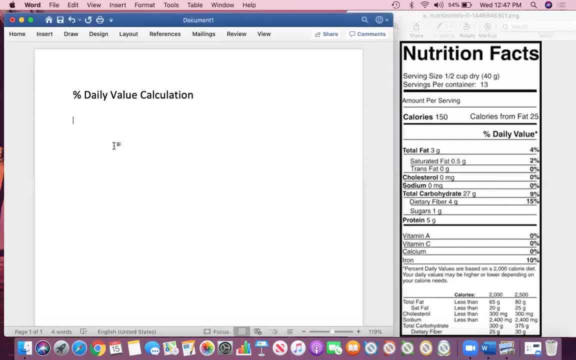 carbohydrates. So, to go over basic percentage calculations, it's going to be the part that you want to calculate over the whole times. 100 equals the percentage. Okay, so in this case the part is the grams of carbohydrates listed on the food label, So it'll be 27 grams of carbohydrate CHO. 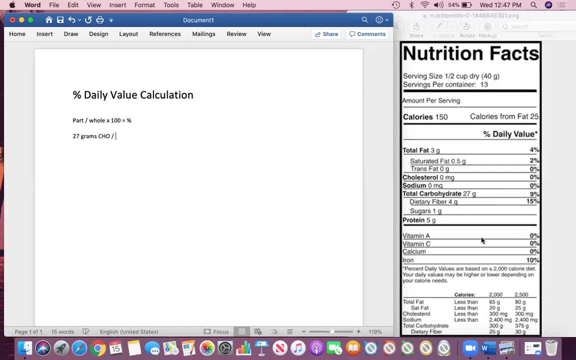 divided by the whole. So in this case the whole would be the total carbohydrates for the entire day, based on a 200 calorie diet. So it'll be 300 grams of carbohydrate. okay, So 300 grams of carbohydrates, so that's for the entire day. So basically, the 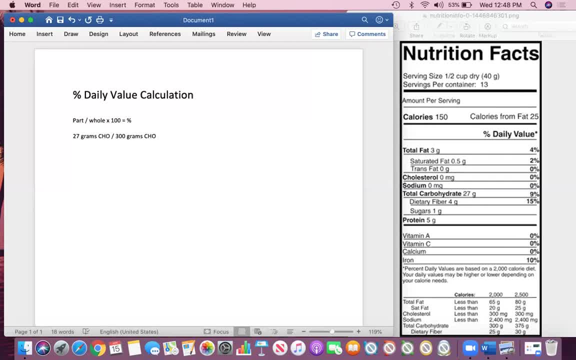 percent daily value tells you what portion of your daily carbohydrate intake you're getting from this specific food. Okay, So you do 27 grams divided by when grams, So that equals the proportion 0.09.. So to make it a percentage, you multiply by 100.